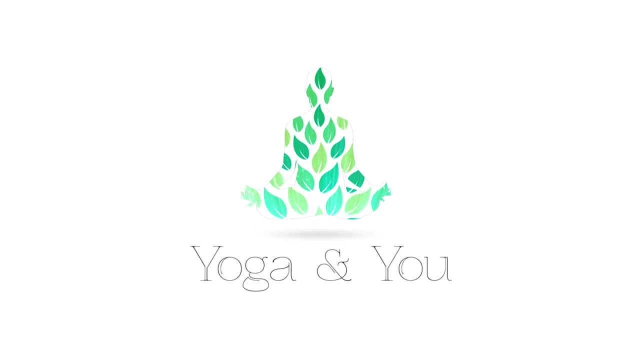 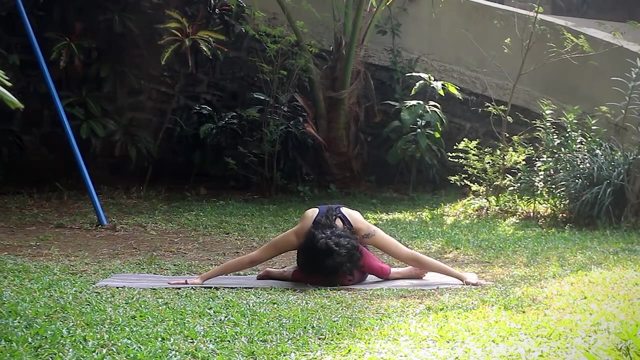 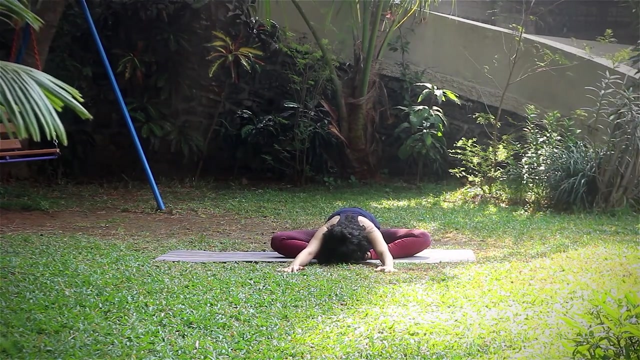 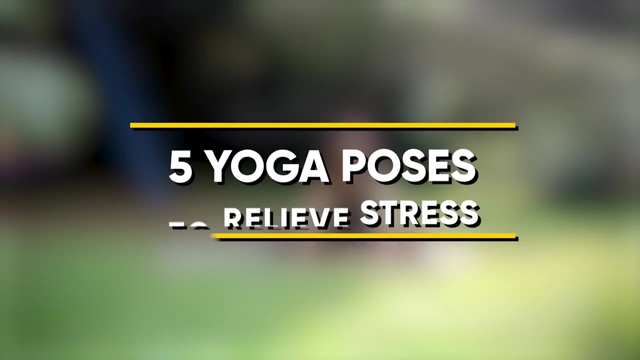 In the middle of a pandemic, it can be hard to escape the feeling of overwhelming stress. Coping with anxiety needs great mental strength. Yoga helps build such strength that will keep you grounded in reality. Here are five yoga poses that will help you deal with stress and retain. 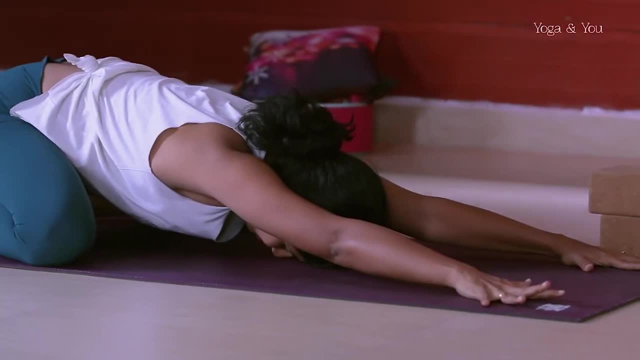 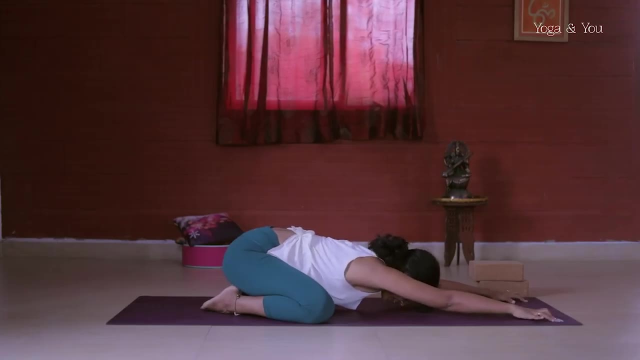 mental balance. Balasana or child's pose. This pose helps alleviate stress and feelings of anxiety. This pose flexes the internal organs of your body and helps in keeping them active. This stretch also helps in the lengthening of the spine and maintaining its natural alignment. 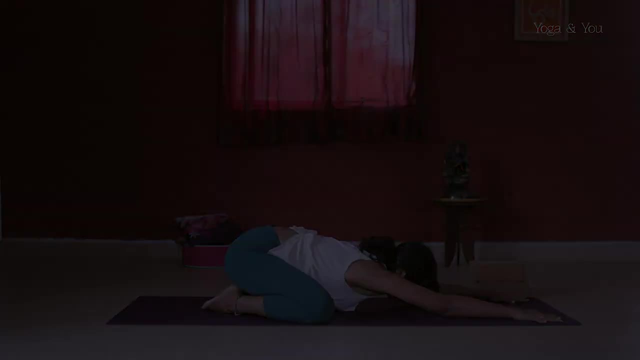 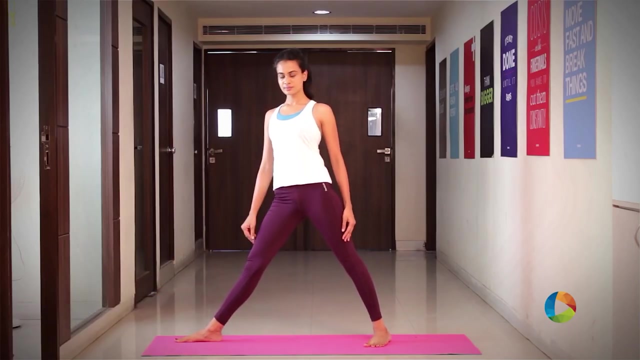 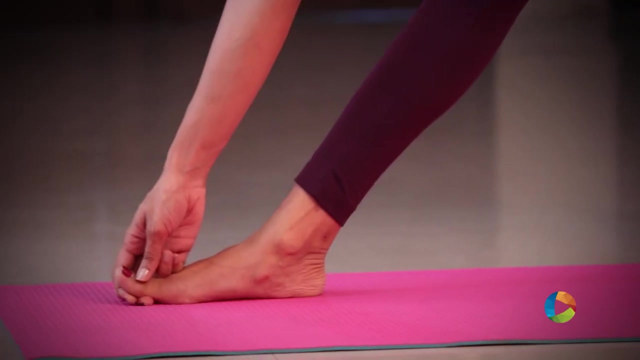 Stay in this pose for as long as you need. Uthita, Trikonasana Uthita, or extended triangle pose. This pose requires balancing your body while taking all the weight at the core. Apart from enhancing the balance of your body, it also brings in 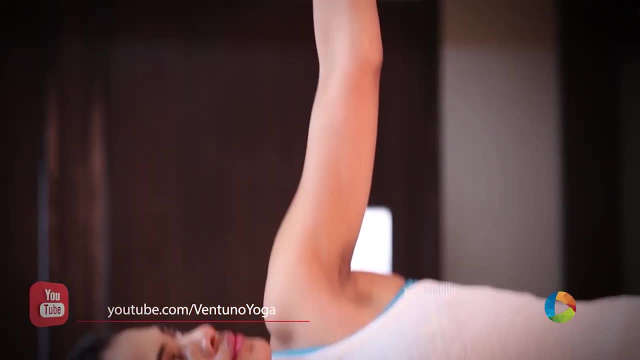 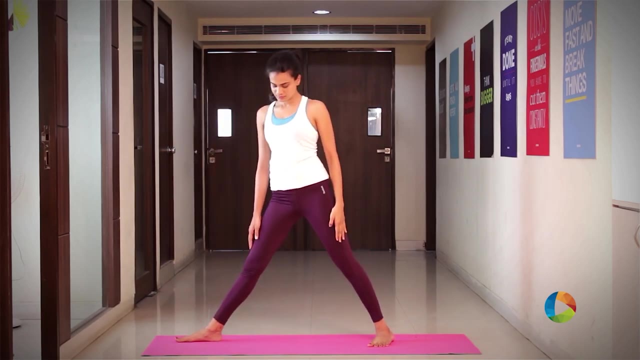 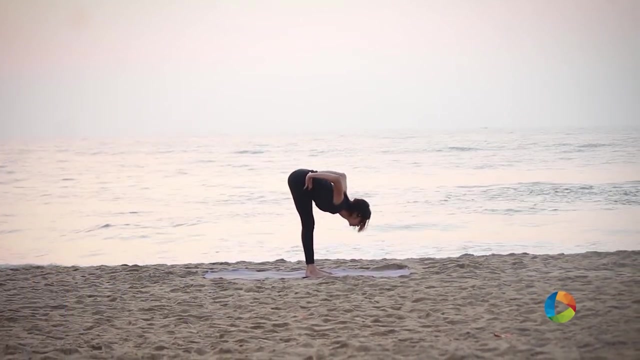 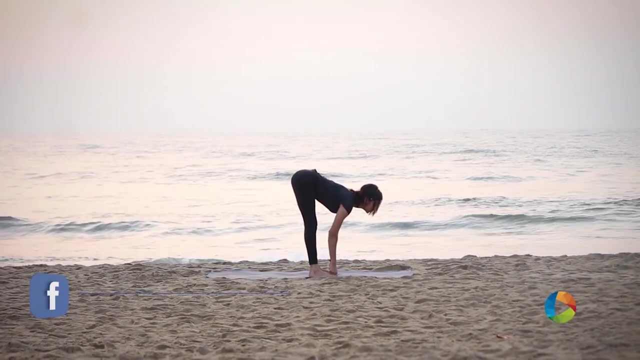 more awareness. Hold this position for 15 to 30 seconds, Breathe in and release your torso, and take a rest in Uthita Tadasana Padangusthasana, or big toe pose. Padangusthasana provides relief from stress, anxiety and tension. It also relaxes the mind, relieves headaches and 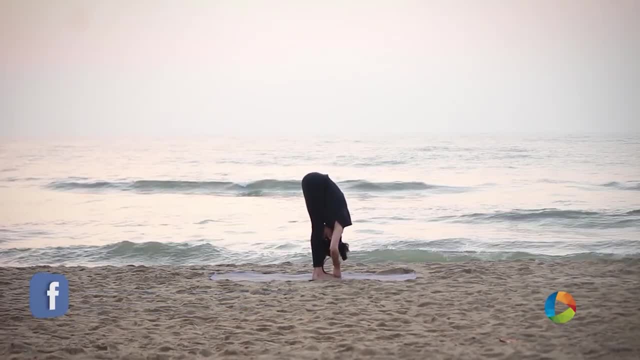 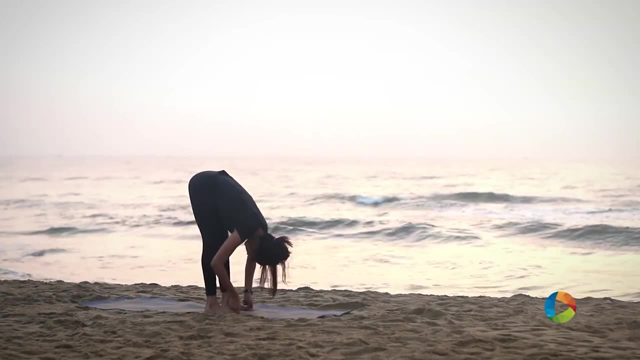 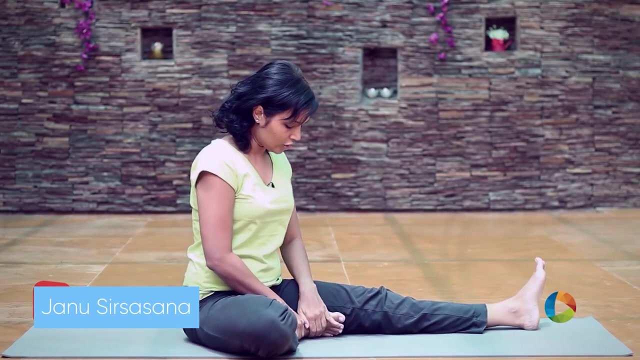 helps deal with insomnia. Keep your torso straight while moving up and down. Hold the final position for one minute With an inhale. swing your torso and head back upright. Janusirasana or head to knee pose. Janusirasana requires both breathing and head to knee bend. 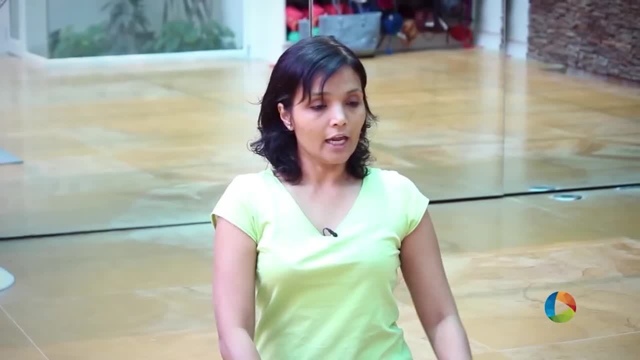 keeping your body in this position for 25 to 30 seconds. Use your手 as a medium for this pose. Pat a little on the neck, fingers on the chest and hands throughout. This also helps in controlling high blood pressure and treating insomnia. 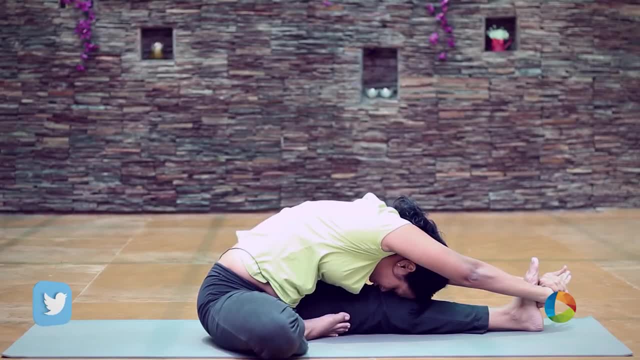 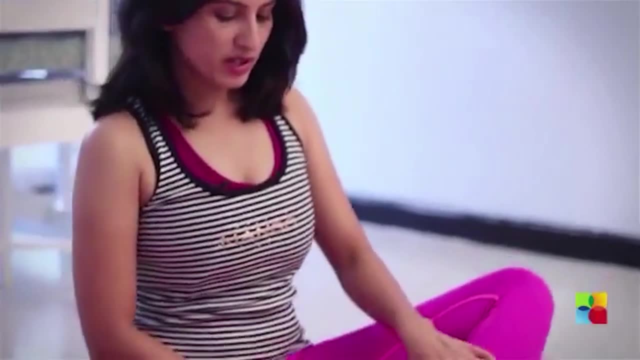 Stay in the pose for one to three minutes, Come up with an inhalation and repeat the instructions with the legs reversed, Sukhasana or cross-legged pose. Sukhasana is the simplest and effective meditative sitting posture that calms your mind and helps you release your stress. 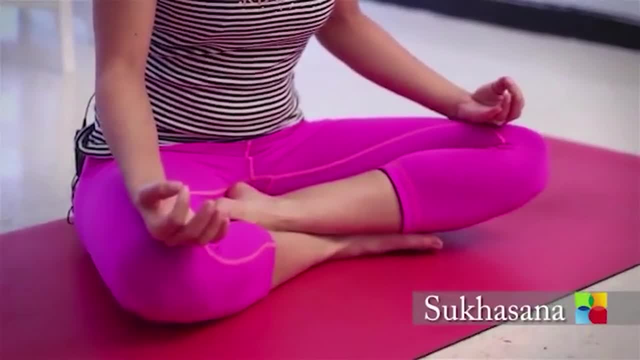 12123. Sukhasana is the simplest and most effective meditative posture that calms your mind and helps you get emotional and fresh. Sukhasana is the simplest and most effective meditative sitting posture that calms your mind and helps you get real energy.